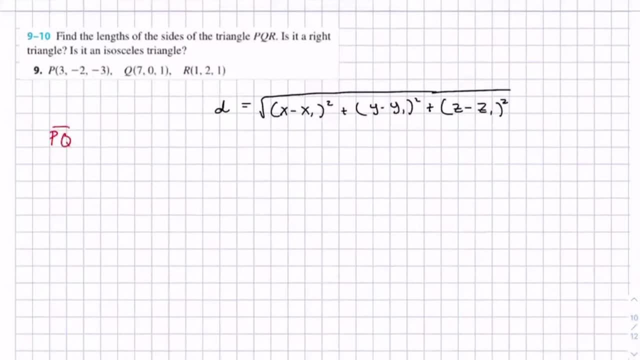 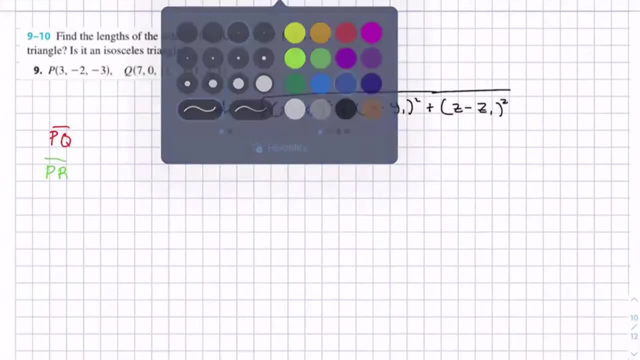 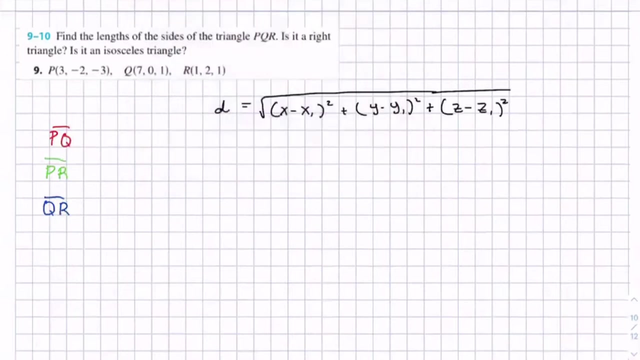 So we have PQ, PR and QR. So this is the three sides of our triangle. So for PQ, D equals 7 minus 3, squared plus 0 minus minus 2, which is plus 2, squared plus 1 minus minus 3, which is plus squared. 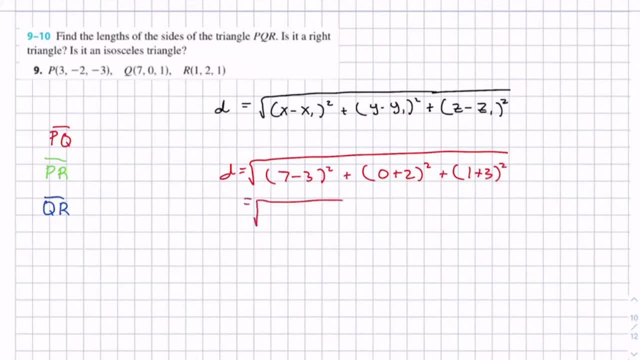 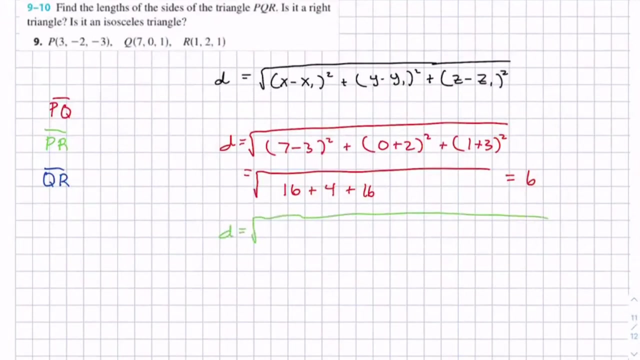 This equals 4 squared, which is 16, plus 2 squared, which is 4, plus 4 squared, which is 16, which is square root of 36,, which equals 6.. All right, so for PR, the distance equals 1 minus 3 squared plus 2 minus minus 2 squared, which is 2 plus 2,. 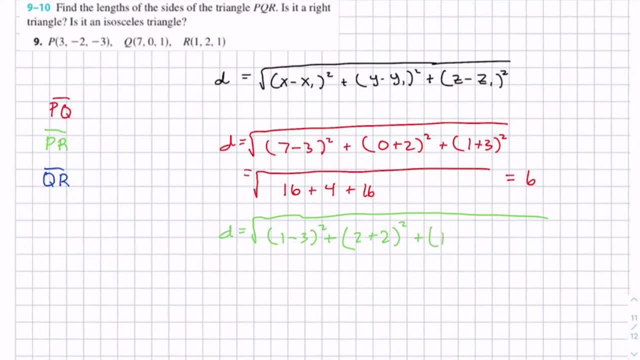 which equals 1 minus minus 3, which is 1 plus 3 squared, And this equals 2 squared, which is 4, plus 4 squared, which is 16, plus 4 squared, which is 16.. 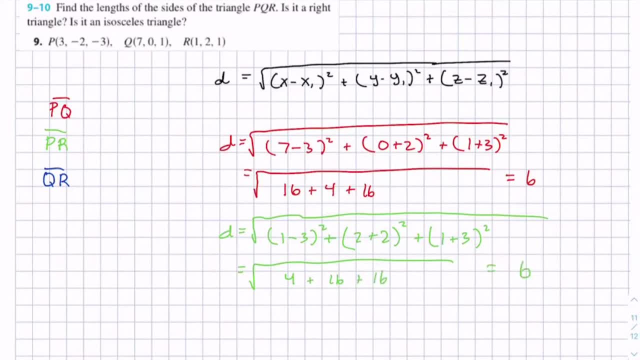 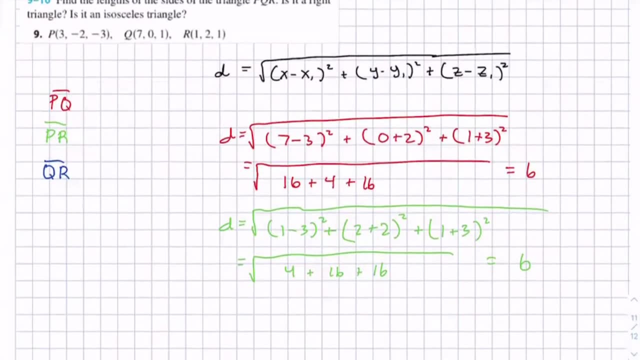 So we have 6.. So we know two of the sides are 6.. But this doesn't yet delineate if it's an isosceles or a right triangle, So we need to go find the last segment, the last side of the triangle, which is QR. 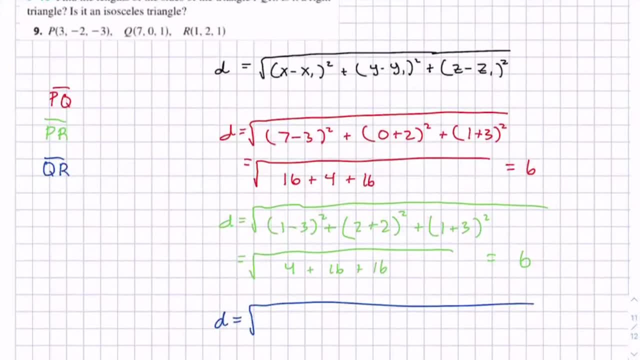 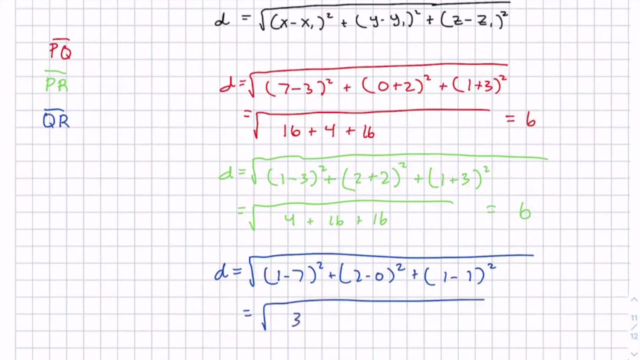 So D equals 1 minus 7 squared, plus 2 minus 0 squared, plus 1 minus 1 squared, And this equals 6 squared, which is 36, plus 2 squared, which is 4, goes square root of 40.. 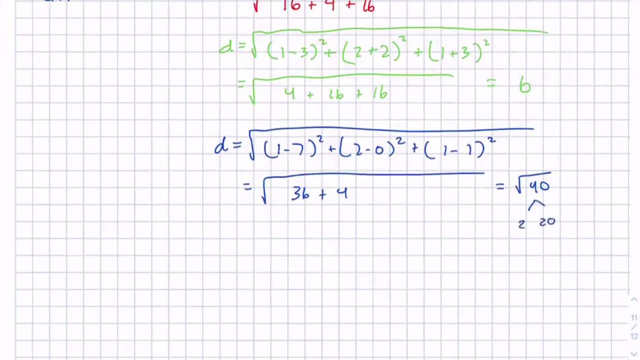 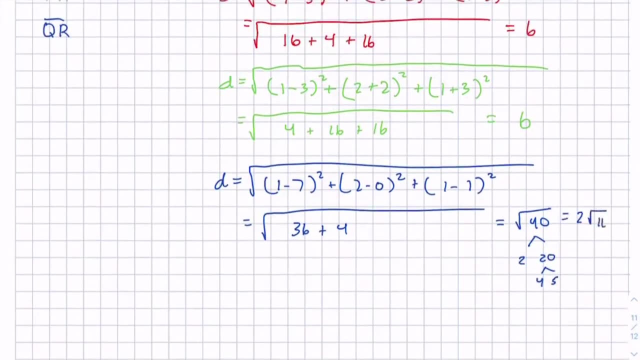 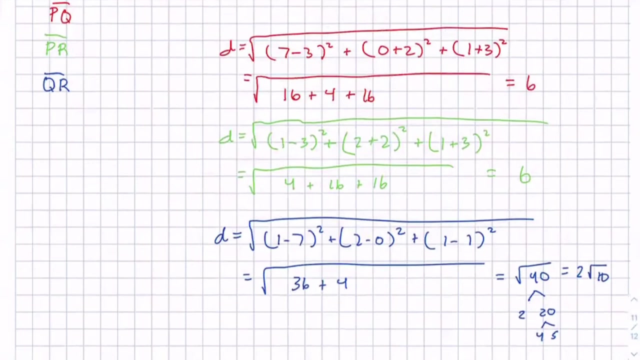 Let's see if you can simplify this at all. So we get 2 and 20,, 4 and 5, so we get 2 root of 10. And you can see that this will form an isosceles triangle.